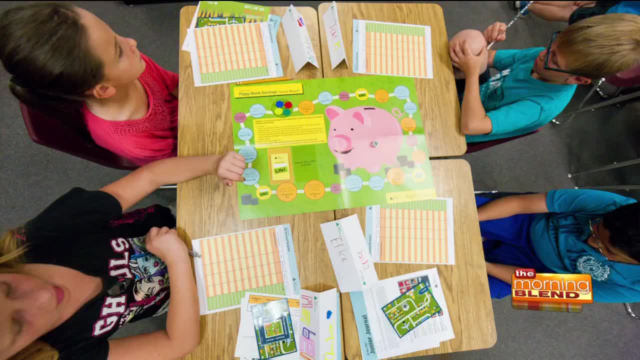 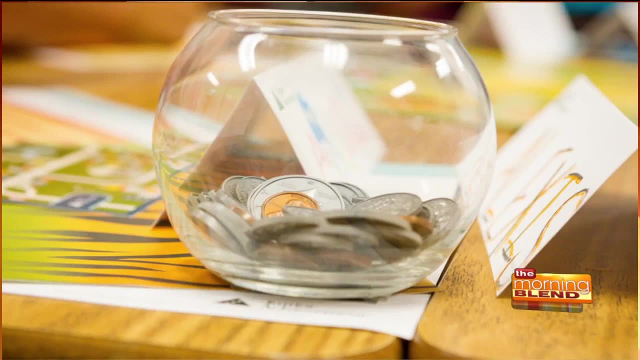 how to do both, And a lot of parents find it difficult to spend. they don't have the resources financially to do everything they want to do at back to school time. So these are fantastic teachable moments that a lot of parents are taking advantage of. have those conversations. 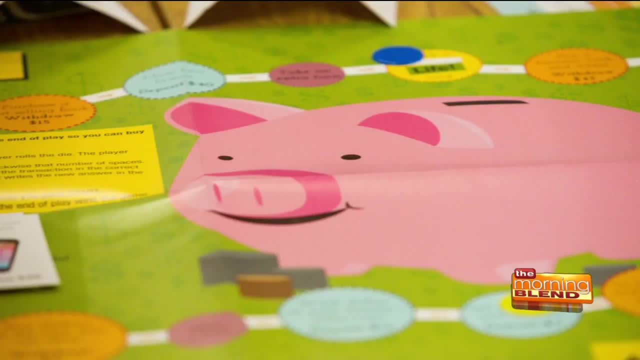 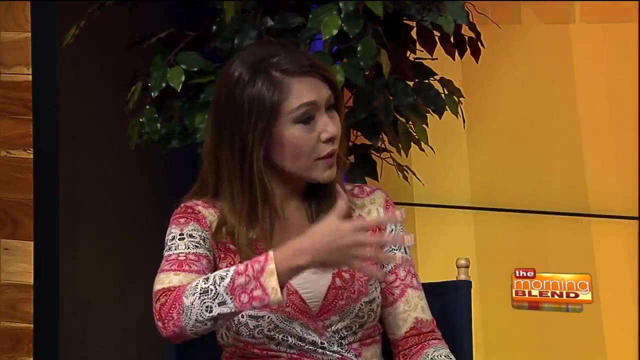 at the store with their children. So it should go beyond just hey, do you like this book? the style of your lunch pail? We're going to turn these into teachable moments And do we have ways we can tell parents to do that? Absolutely, Especially with older kids, but younger kids. 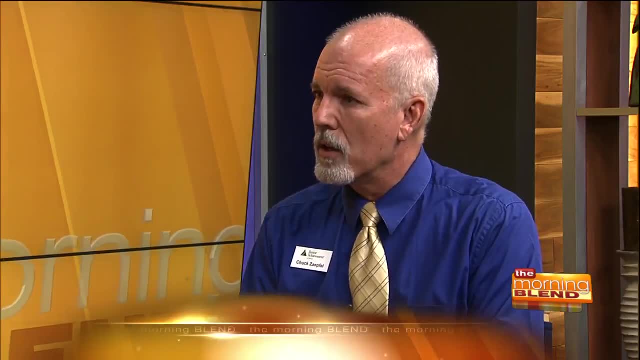 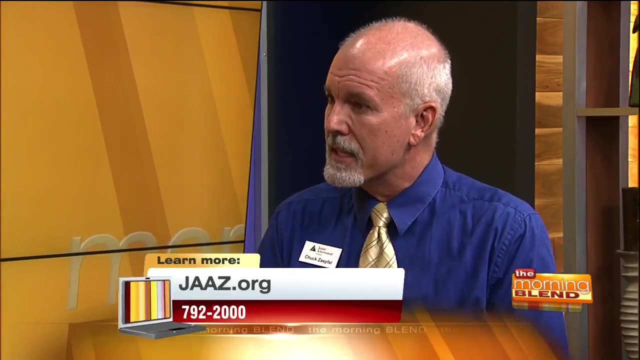 too. We can talk about that when you're buying clothing or shoes. I mean, you may want Nikes, but you need shoes. So it's under the terms of who wants and needs. Involve them in the decisions, because learning to spend, whether they want the higher end binder versus the lower end. 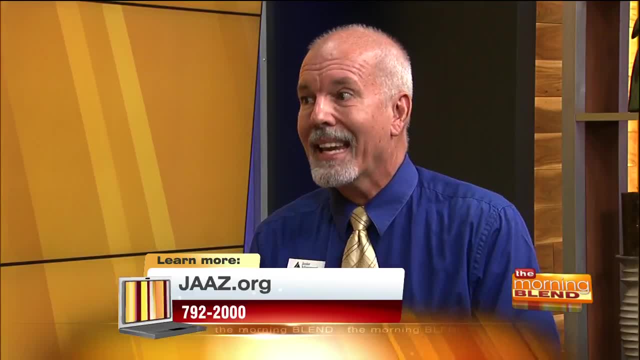 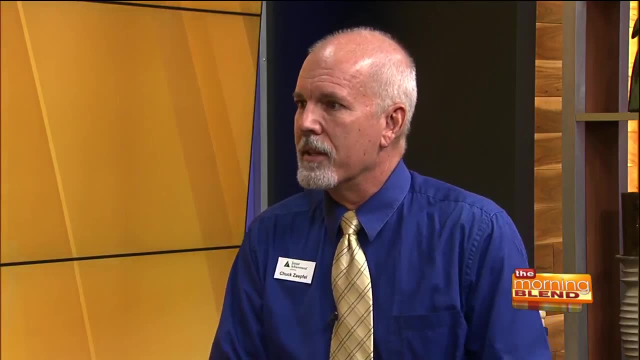 means that we can buy other things that you do want or need at the same time. So having a conversation and that shopping experience is helping them grow Up to be responsible adults and be able to teach their children- And I've said this about junior achievement Every time we've talked about you guys on the show. 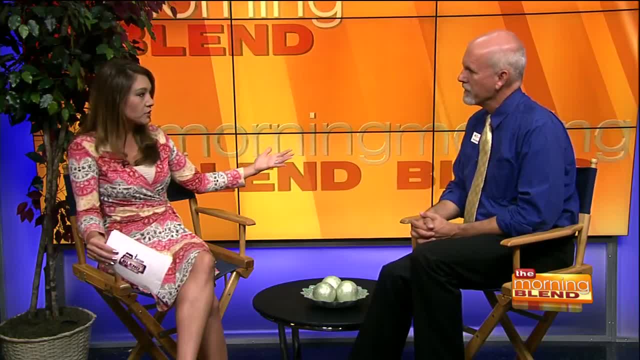 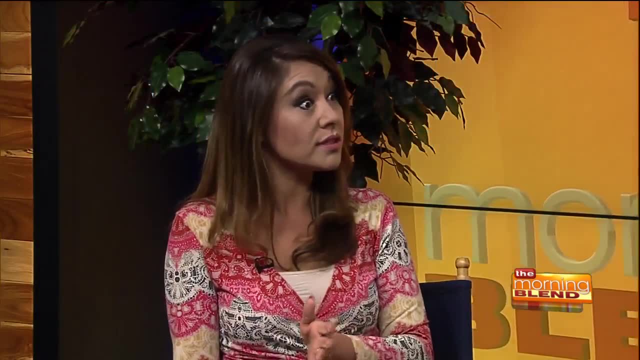 I wish that this type of a program was available to me when I was younger, because these are real life lessons And we're kind of taking what you guys do in your program and saying: hey, parents, you can also do these in these everyday, routine things. So what are some of? 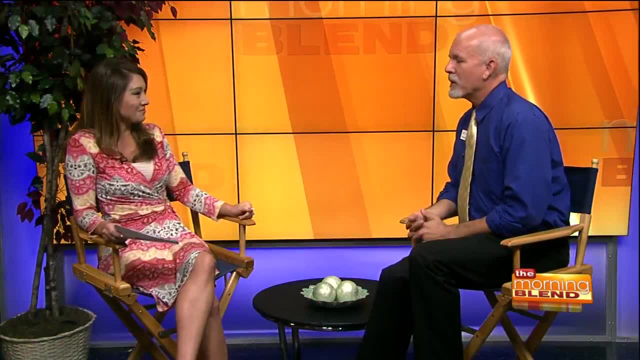 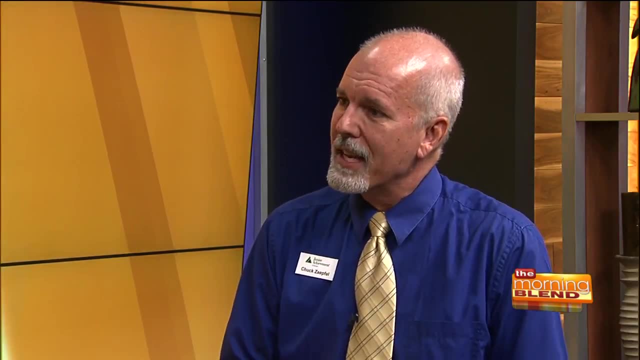 the other ways that we're doing those teachable moments for students. Parents have a lot of places they can do that: If they're at a restaurant, when they're in the grocery store. I always took my kids grocery shopping to have those conversations Sometimes. do you want to get generic? Do you want to get the name? 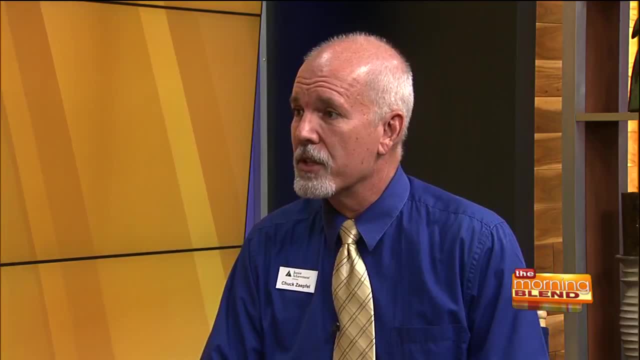 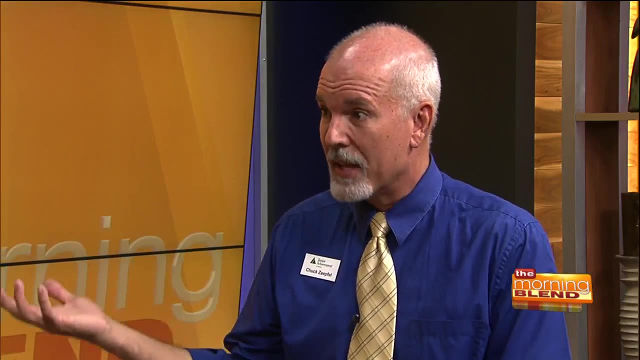 brand. How much do we want to do If we're going to have friends over? those conversations are great teachable moments for them. For junior achievement, we're teaching a lot of these same things And we're reinforcing what the classroom is teaching them, what the parents 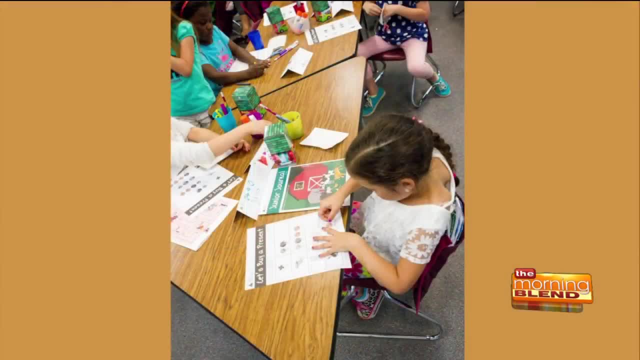 are teaching them, but from our volunteers in the classroom sharing that again. So they give the message from a lot of different ways And it is- I think it's- a round. What do you mean? a little bit at home, We've got some at school And you kind of absorb all that, And then of 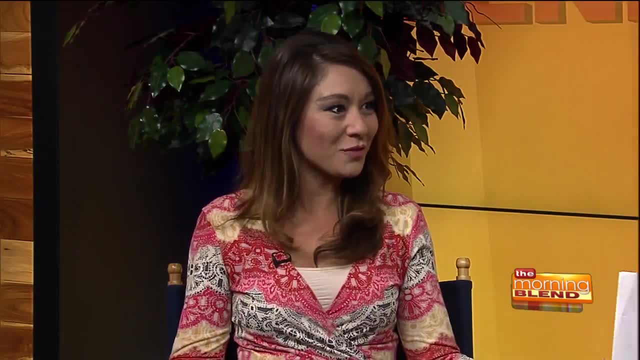 course, as you become a student, you kind of absorb all that And then, of course, as you become a an adult, you're like: whoa, this stuff is real life things I could use, And that's really what.